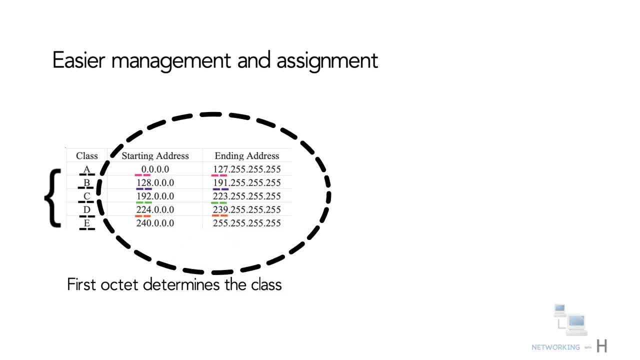 determines the class D IP address range and the last, 240 to 255, determines the class E address range. IP addresses from the first three classes, A, B and C, can be used for the host addresses. The other two classes are used for other purposes. 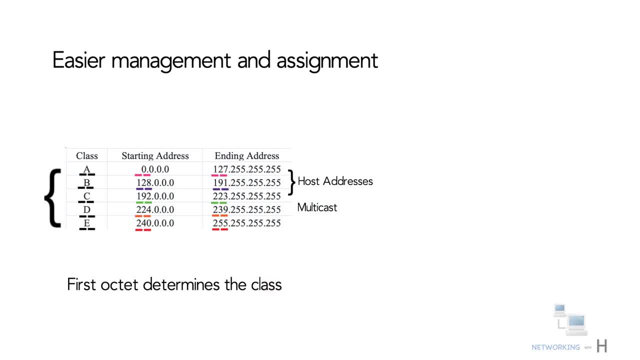 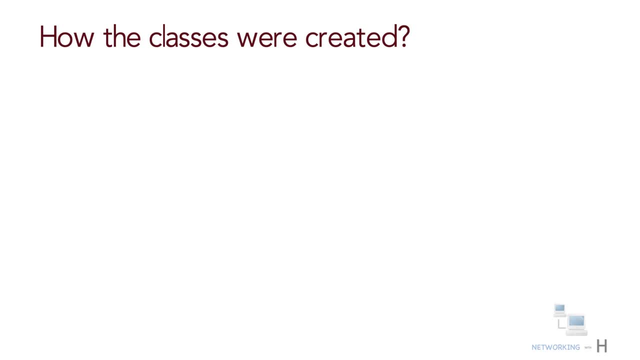 Class D for multicast and class E for experimental purposes. Let's see how the classes were created. As you know, an IP address is the combination of network and host ID. In each IP address, few bits are reserved for network address. The classes were created based on the network size. 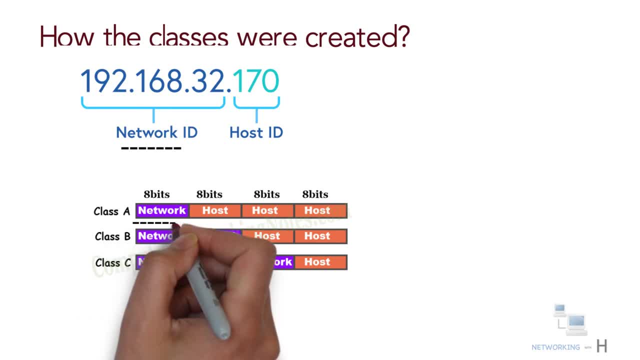 In class A, the first eight bits are reserved respectively for network addresses which gives you to subnet mask of slash 8 or 255.0.0.0.. In class B, the first 16 bits are reserved respectively for network addresses which gives you the subnet mask of slash 16 or 255.255.0.0.. In class C, the first 24 bits are: 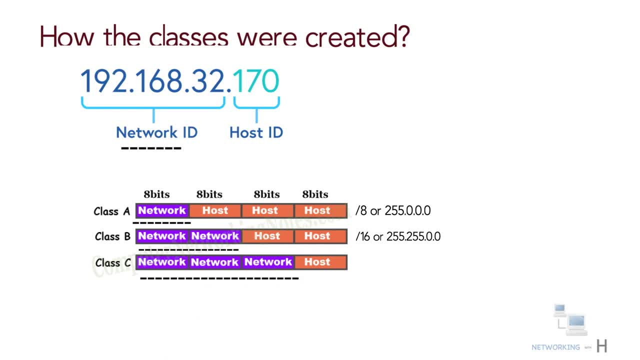 reserved respectively for network addresses, addresses which gives you the subnet mask of slash, 24 or 255 or 255 or 255.0.. For example, for the small number of networks with a large number of hosts, the class A was created. 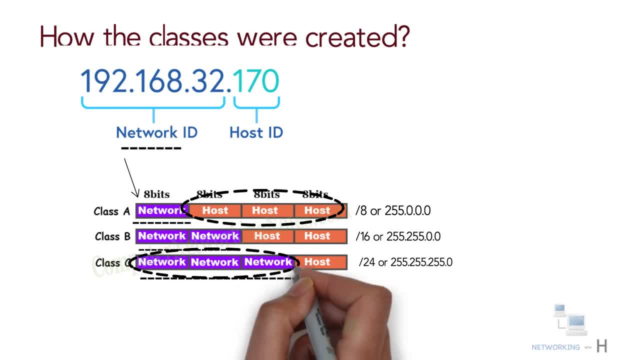 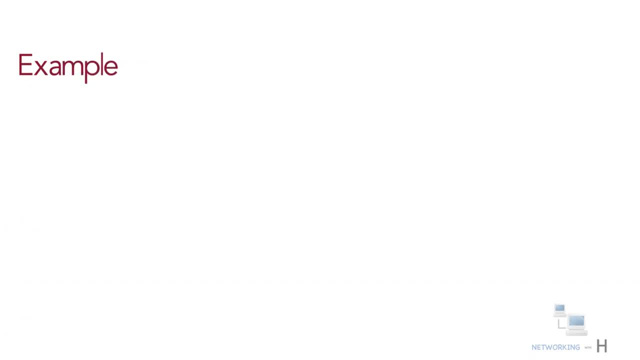 The class C was created for numerous network with small number of hosts. Let's use an example to find the class of three different IP addresses: 192.168.1.1.. To find the class of an IP address, simply pay attention on the first octet. 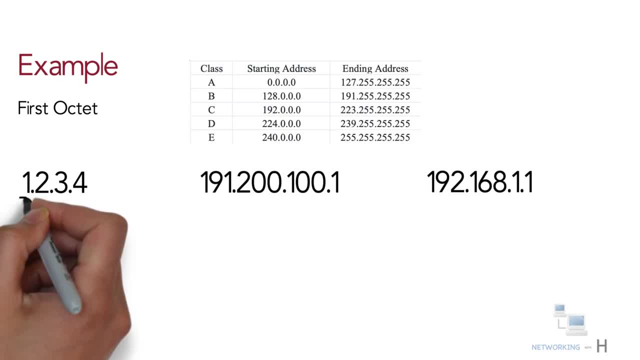 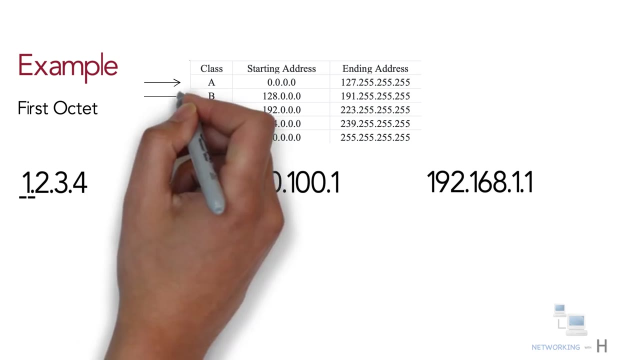 Let's start with 1.2.3.4.. If the value of the first octet is in the range of 1 to 127, you can say it's a class A IP address. If the value of the first octet is in the range of 128 to 191, it's a class B IP address.